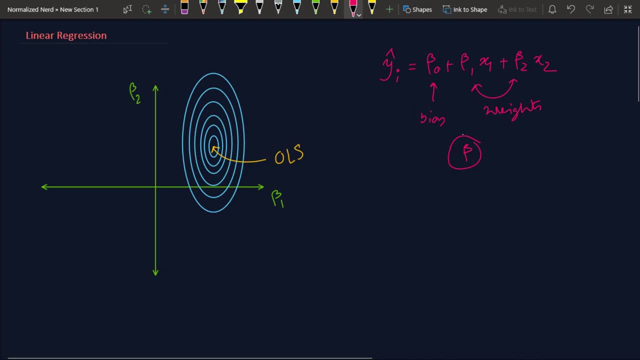 parameter. All right, And when I talk about weights, please remember that I'm talking about only beta 1 and beta 2, and when i'm talking about bias, i'm talking about only beta 0.. okay, got it. so? uh, this is our model and to apply ordinary least square method, we have to define a 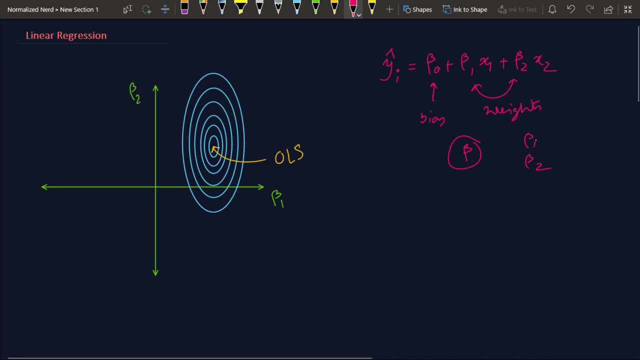 cost function and i hope that many of you are familiar with the cost function, that is, least square cost function, and the formula goes something like this: j of beta and it is equal to 1 upon 2n. by the way, n is the number of data points in our data set. 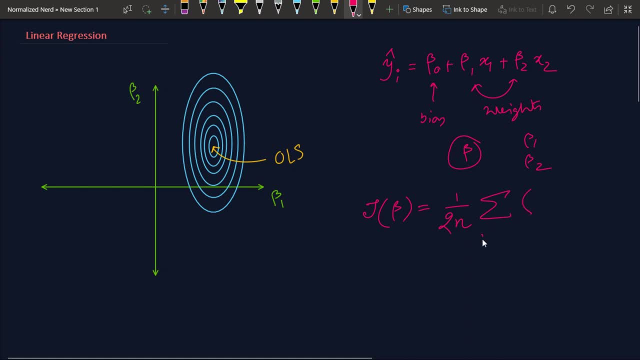 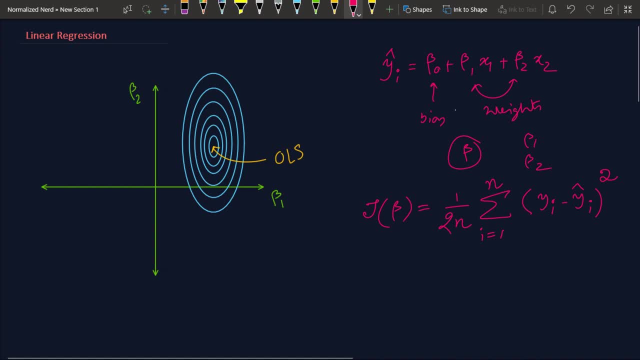 to get the values of beta. okay. so i have drawn here a contour plot of this function and you can see that i have drawn only the beta 1 and beta 2, that is the weights, and i have discarded the beta 0. that is the bias, because throughout the analysis i really don't need bias term. okay. 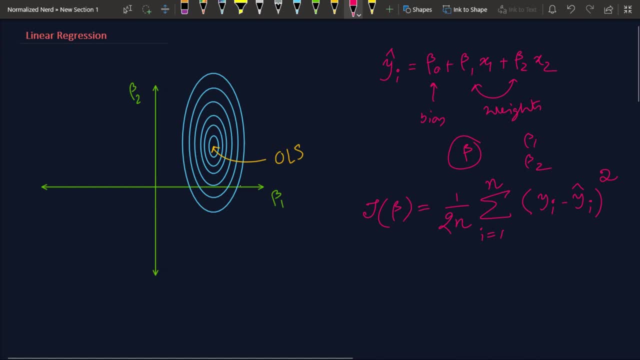 so here is the contour plot, and i hope you know that contour plot simply represents higher dimensional function into a lower dimensional plane. that is, here we have a 3d function represented in 2d plane, all right, and every point on this concentric circle corresponds to the same height. okay, so we are good to go. 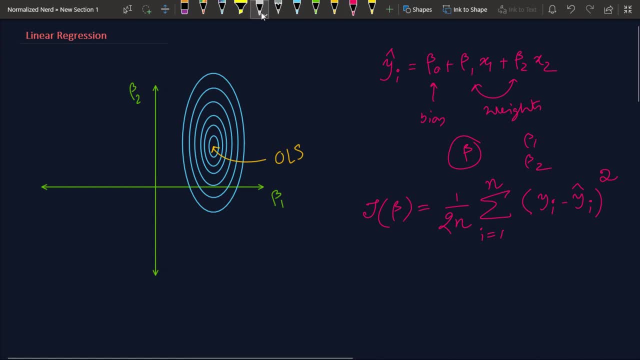 and here i have pointed this particular point, which just represents the minima of this function. so after the minimization we will find the weights, that is, beta 1 and beta 2, here. so in vector space we can just represent this- two values- using one point. all right, so imagine we are drawing an vector from 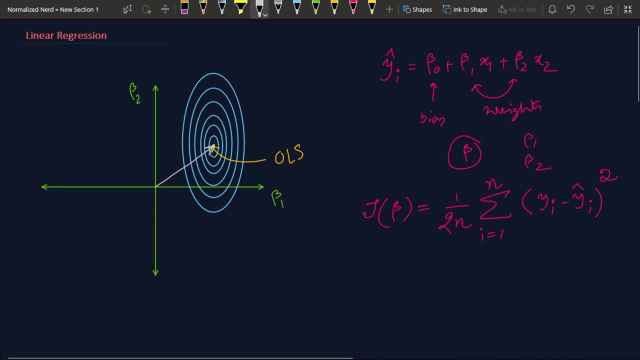 here to here. so this: if I just drop perpendicular here, so this is our beta 1, and if I drop perpendicular here, this is just beta 2, so that's how we represent a vector in vector space. so after the minimization, our vector of weights beta will be this. so that was all about ordinary least square method. 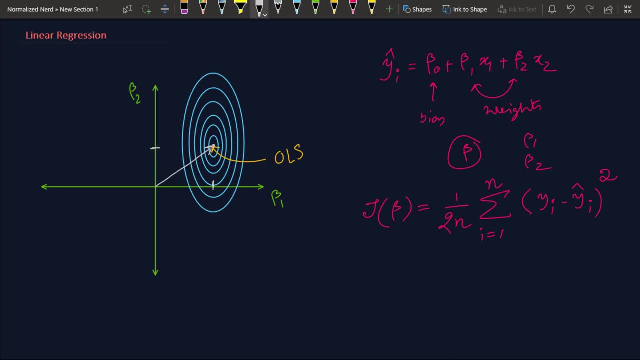 but here we have a huge disadvantage, and that is overfitting. well, I'm not really gonna explain all the caveats of overfitting, but I'm just gonna give you the gist. well, overfitting simply means our model has learned our training dataset so well that it fails to generalize on unseen data. well, the main. 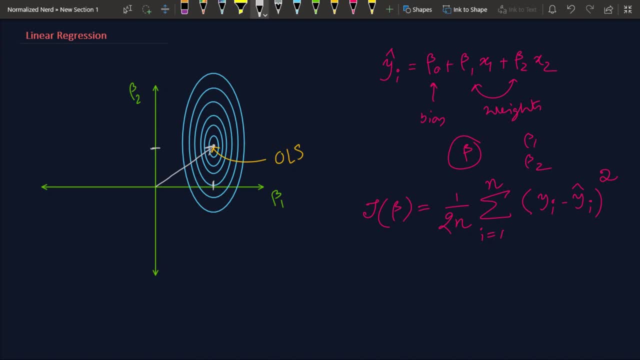 reason behind overfitting is that our model has learned tiny variations, which are insignificant, but our model has learned the tiny variations in our training set, and this happens when some of the weights are very, very large compared to the others, in other words, when we assign too much. 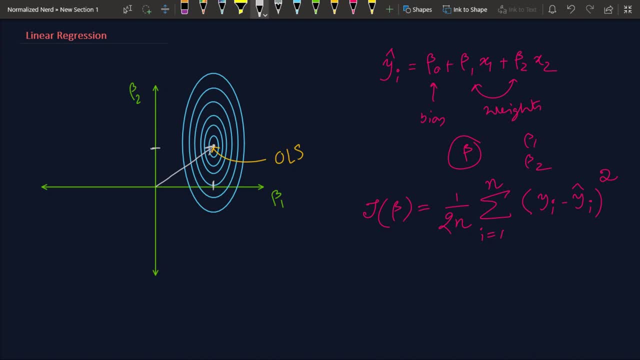 importance to some features compared to the others, the model tends to overfit. now to tackle this problem, we have actually many methods available, but to show you the different kinds of linear regression, we just need to talk about only one method, that is the regularization. now to regularize our 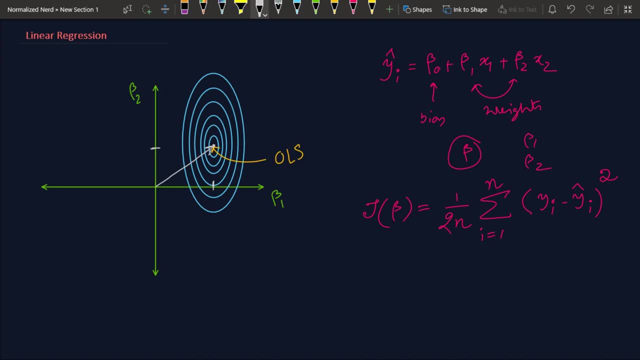 model. we just need to add one term to our cost function. this is our cost function, right, and by adding something, something with this, we will gonna get a new cost function, and that will be our new model. well, what we should put here? there are actually two famous choices. the first one is adding the sum of the squares of the 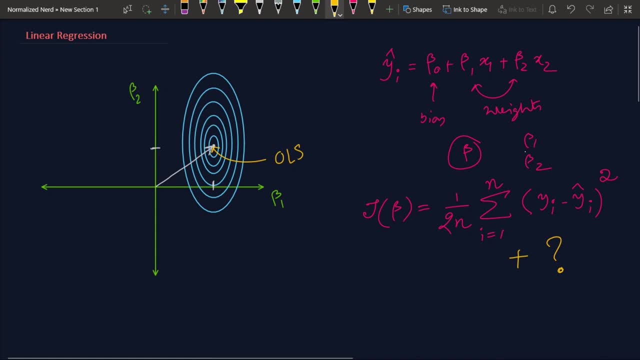 weights, and that is termed as ridge regression, and in the other case we add the absolute values of our weights. okay, which is called as lasso. first I'm gonna show you the cost function of ridge regression, and the cost function goes something like this: don't focus on this plot now, because I will explain it to you in a minute. 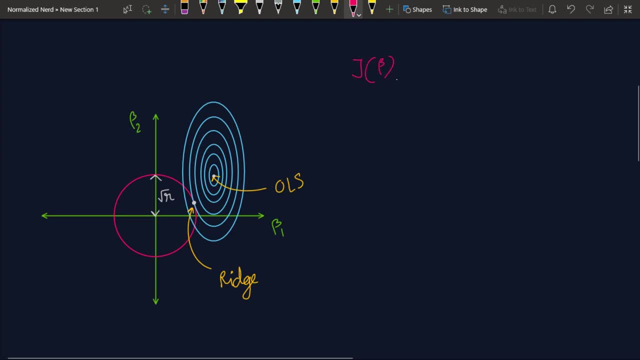 later. so here I'm just writing R as ridge. it is equal to well. the same thing I have to write again. plus we are adding here beta j2. now notice here two things. the first one is we have another coefficient called lambda here, and we have started the summation from one. but if you noticed, 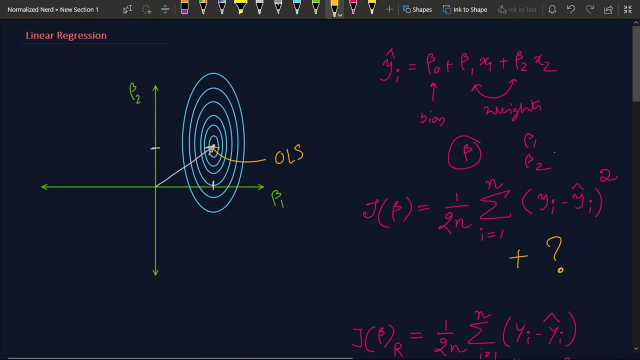 here they're, the beta. start from zero. but, as I have told earlier, that bias term is not going to be important in our analysis, because overfitting happens mainly due to extraordinarily large values for the weights. So we just need to regularize our weights, not. 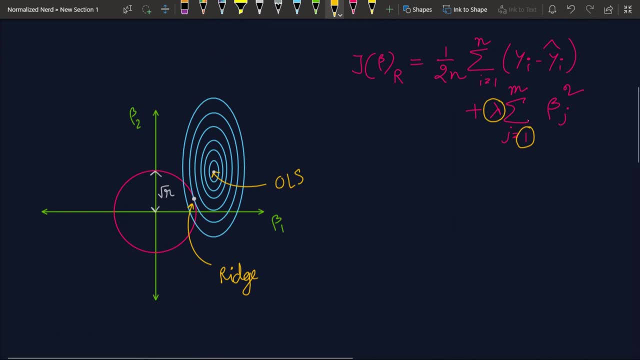 the bias term. That's why I have started this summation from 1 and m is just the dimension of beta. So here's the cost function of ridge regression. but this equation doesn't tell you much about this concept and it doesn't really give you any intuition. Better if we can write. 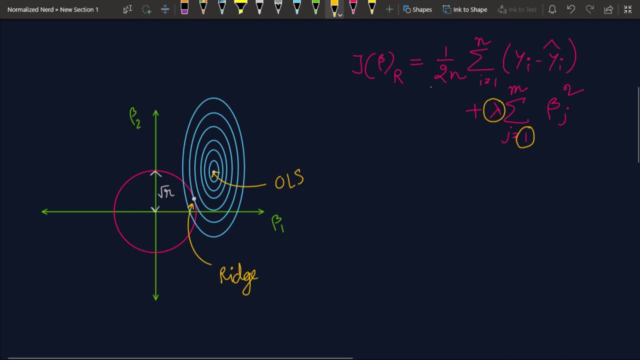 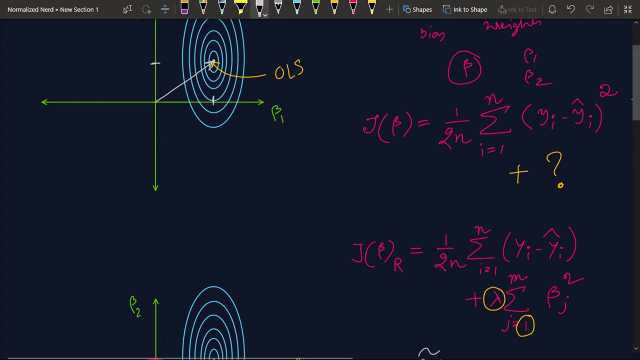 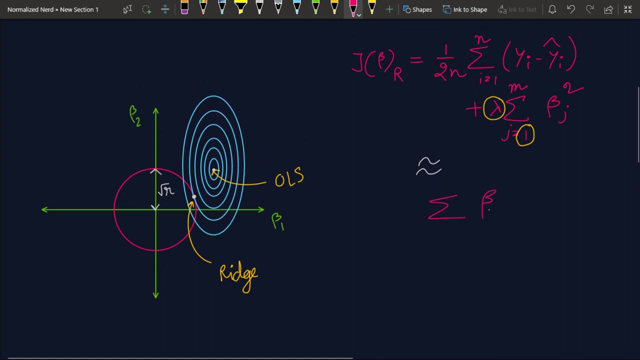 it in some different format, and the format I am interested here is this: equation is equivalent to minimizing our previous function with a function Additional constraint. and what is the constraint? Well, the constraint is simply the summation of beta- j. I am dropping the j and m here, just for simplicity. square must be lesser equal to some. 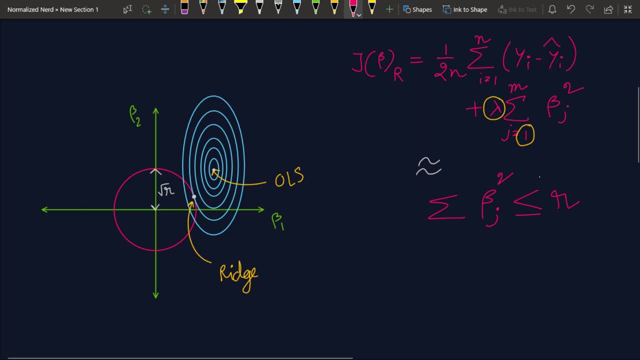 positive value r. Now it can be proved that for every lambda there exists a positive r. That's why this equation is equivalent to minimizing our previous equation under this constraint. Now focus on this plot. Well, this constraint can be visualized as a circle here. The center of that circle is the origin. 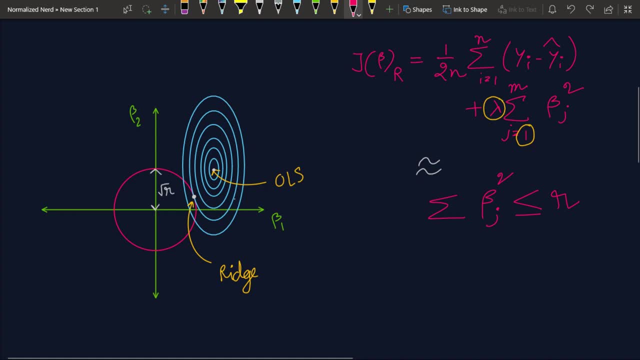 all right, and previously the beta was converging at the minima of our contour of the cost function. but now the final value of beta we will get here, because this constraint doesn't allow our beta to go outside of this red perimeter. isn't it amazing that we can visualize this? 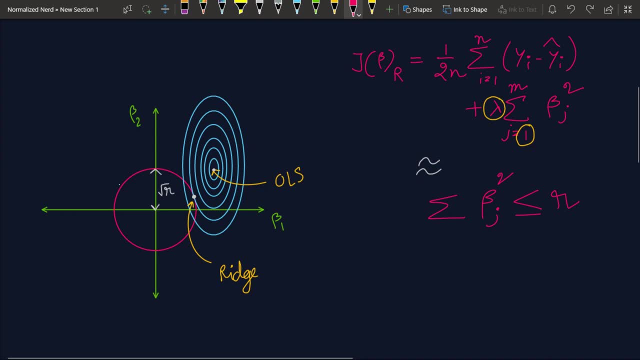 equation by this intuitive plot. i think it's amazing. and now you should be asking yourself: why does it prevent overfitting? if you look closely here, as we increase the value of beta j's, this term actually increase, but we have to minimize this term so intuitively. 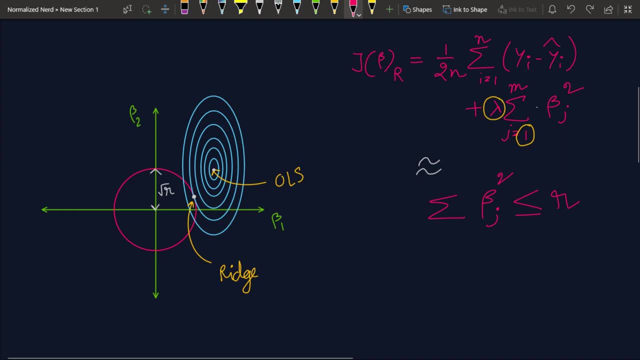 we cannot increase our beta indefinitely. there must be a value after which we cannot increase our beta, and that's what the constraint is all about. the constraint is that we cannot increase our beta indefinitely, so we cannot increase our beta indefinitely. so we cannot increase our beta indefinitely. so we cannot increase our beta indefinitely. 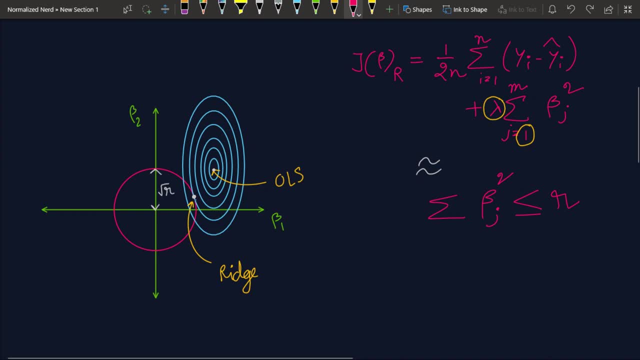 is restricting the values of beta closer to the origin, and this means no feature will get too much importance than the other features. that's how we are tackling the problem of overfitting here. now i'm going to show you something called lasso regression. well, here, 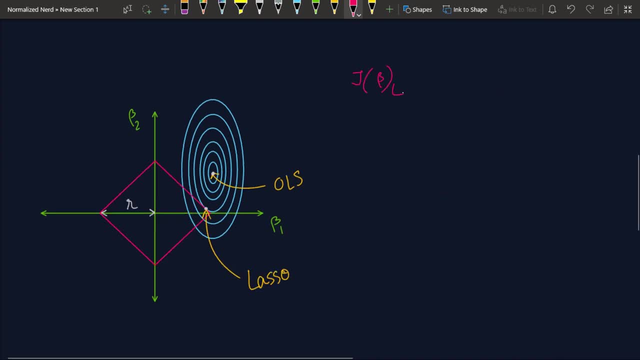 the regularization terms look something like this: i'm dropping this i and n here, also squared. plus, here comes lambda summation over the beta j's absolute value. all right, we are not using the squared term here, but we are using the absolute value, and this is equivalent to: 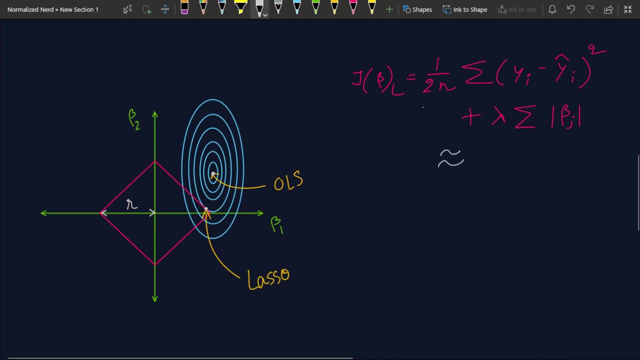 the absolute value of beta j's absolute value. all right, we are not using the squared term here, but we are not using the squared term here. but we are not using the squared term here, but we are minimizing our original least square cost function under the constrained summation of beta j's must be lesser, equal to a positive number and again we can find an positive. 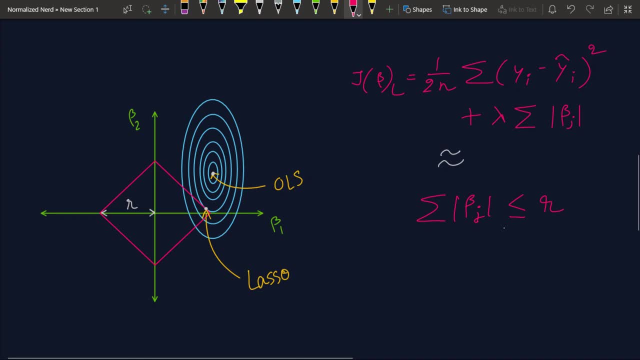 r for every value of lambda, and you guessed it right that this can be again intuitively explained by this plot. so this in equation can be represented by this square and similar to the ridge regression. we cannot move our beta outside of the square, so here the final beta lies, here. 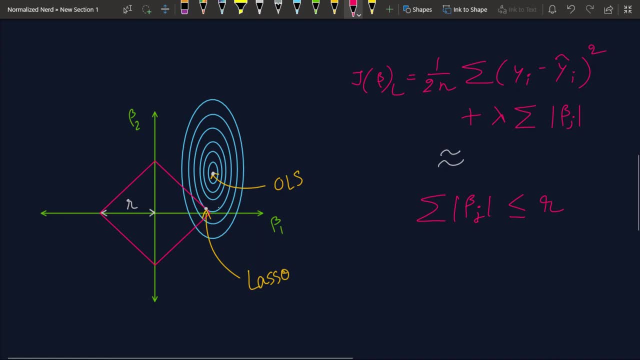 now, there's a very interesting thing about lasso regression, that is, it can automatically select features. how does that happen? suppose our contours look something like this. let me draw another contour here. forget about the previous contour, now focus on this contour. what will be the final result of? 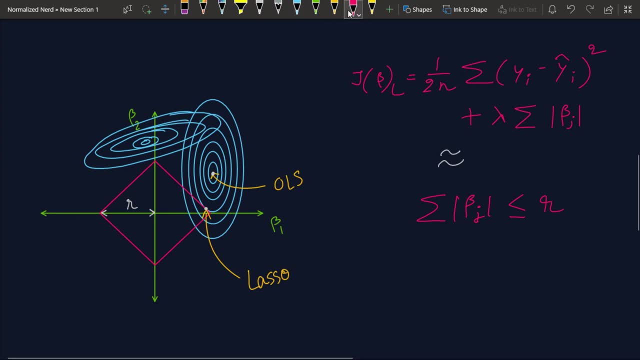 beta here. well, you can see that, as beta cannot move outside of this red square, so the final value of beta should be this: well, this simply means that we have beta r1 equal to 0, so we are automatically discarding the feature x1. all right, and suppose we have 10 features, so we'll have a. 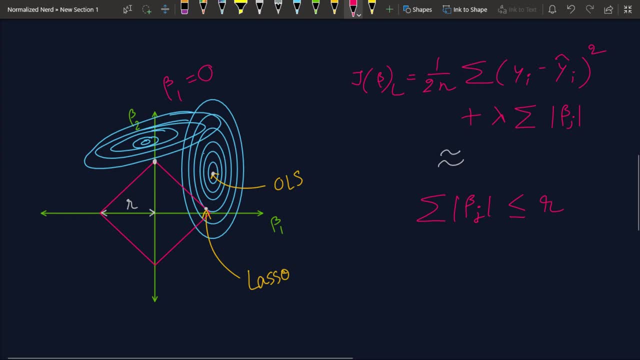 multi-dimensional diamond. and if our final feature x1 is 0, then we have a multi-dimensional diamond. and if our final final feature x1 is 0, then we have a multi-dimensional diamond. and if our final value of beta falls on this axis, so we are just gonna neglect the other axis. so 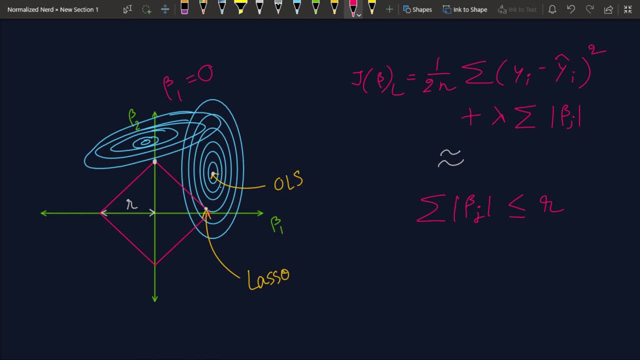 that's how lasso can be used as a automatic feature selection model. now I would like to introduce some side notes here that might be helpful for some of you. suppose we are increasing the value of lambda. what will be the effect on our cost function? well, as we are increasing the value of lambda, we 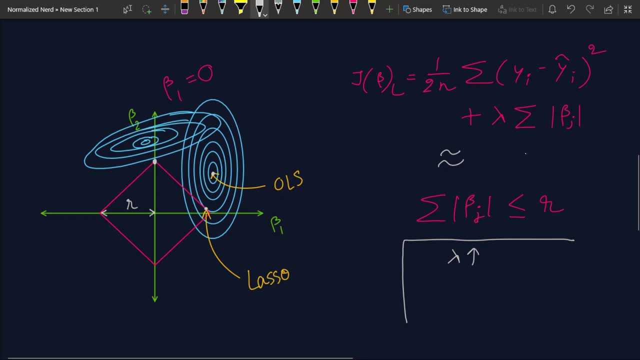 are constraining more and more on our beta j, so the bias in our model will increase and our model will not learn the minute details in our training set. so ultimately it will result in under fitting. and what if we just use a little lower value of lambda? well, if we just decrease the lambda, then we are actually 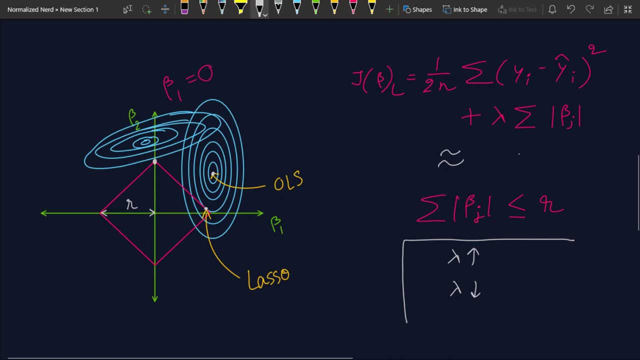 reducing our constraint and it will tend to learn the minute details in our data set. all right, what if we put lambda equal to 0? well, if we put lambda equal to 0 in either lasso or in ridge, we will find just our ordinary least square. 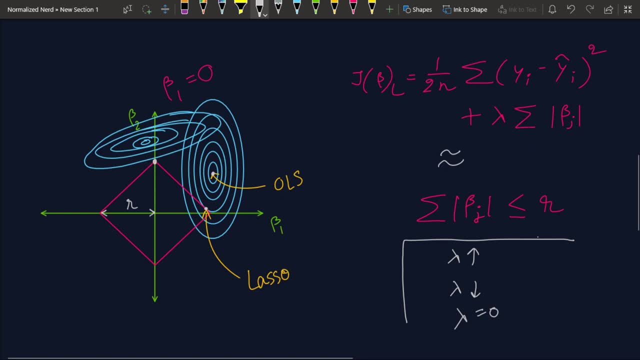 method all right, and I can't just tell you the correct value of lambda for your model because it depends on the data set. so you have to find the correct value of lambda for your own problem and generally it lies between 0.1 to 0.0001. 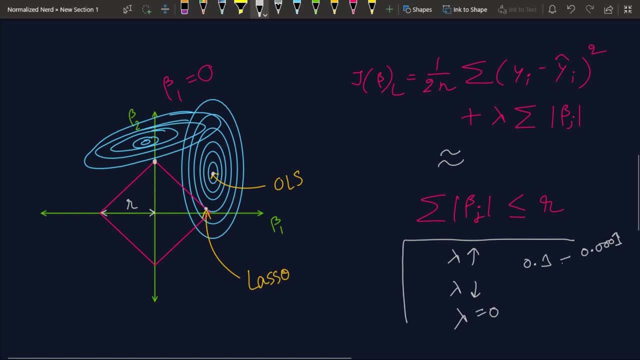 so was that it? have we just covered every possible linear regression model? well, not quite yet. what if we want to use something different in place of this term? you can see that in these three models, we are just using this difference between ground truth and the prediction value as our error, and this is called. 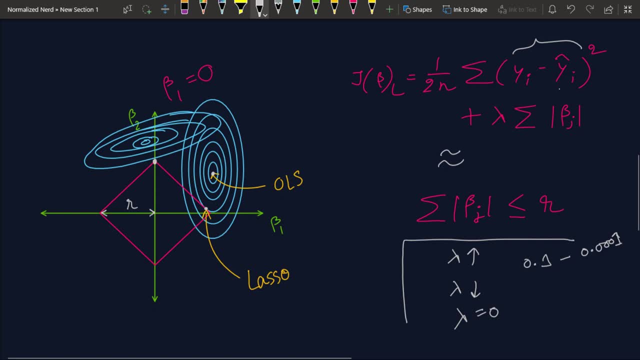 residual and we are just squaring them. what if we want to use some different kind of residual now? why would anyone want to do that? I'm gonna explain that towards the end of this video, but for now let's explore what are the different possibilities for our residuals. first, 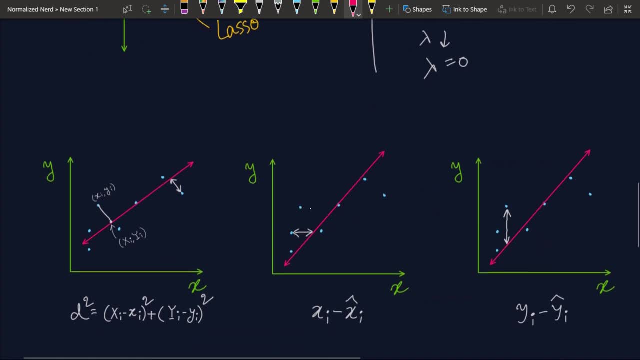 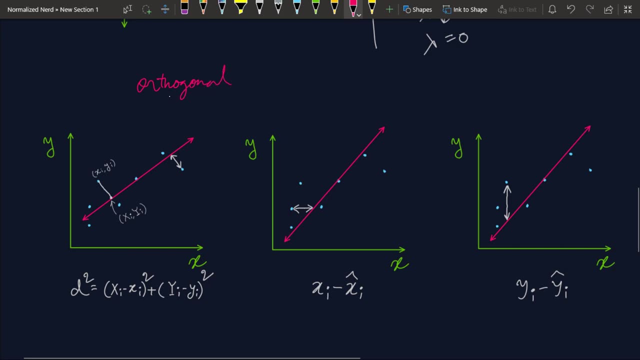 I'm gonna show you something called major axis regression or orthogonal regression. this is the thing, and here we consider the squared distance between the ground truths to the best fit line as our residual. and here you can see that this is our ground truth point and we have drawn a perpendicular to the best fit line and obviously this angle. 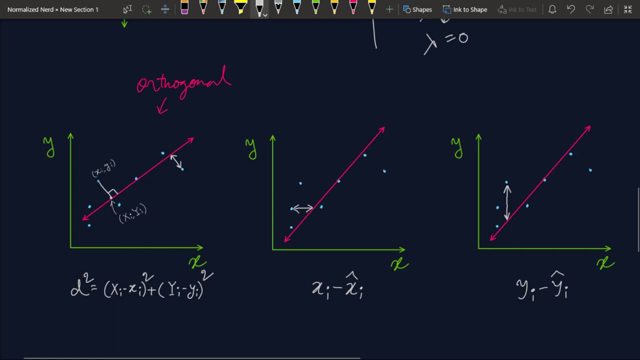 is 90 degree and this line, the length of this line is D and we are squaring this and by Pythagorean theorem we can easily find this and we minimize this D square. so instead we are going to use this D square and this is a square and this is a. 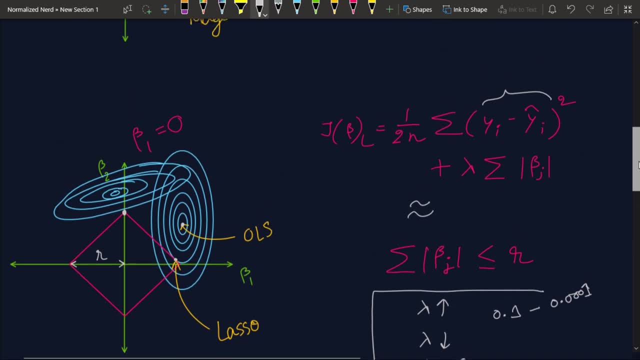 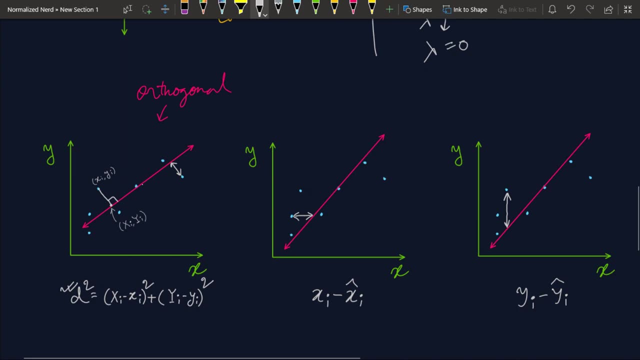 square, and this is a straight line, and this is a normal line and this is a. Instead of minimizing this term, we minimize the d squared term. Now, just to give you a sense how it is different from our above three methods, look at these two plots. 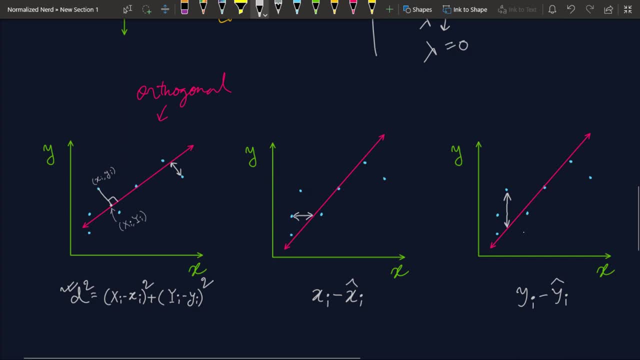 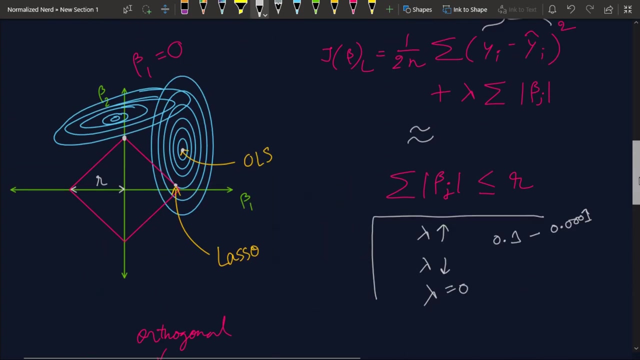 Well, this is the most common plot, I think, and you see here that this distance is just yi minus yi squared, which simply means the difference between ground truths and the predicted values, and this term is actually same as this. However, we could have also done like this. 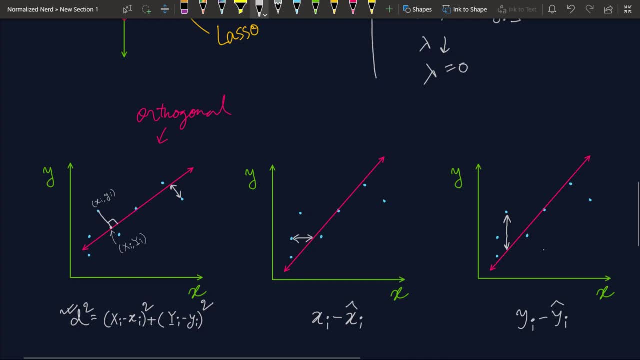 Here we are considering the error along x-axis, but here we were considering the error along y-axis, but in this case we are considering the error that is in the perpendicular direction. so in a sense, in this orthogonal regression we are actually considering the errors in. 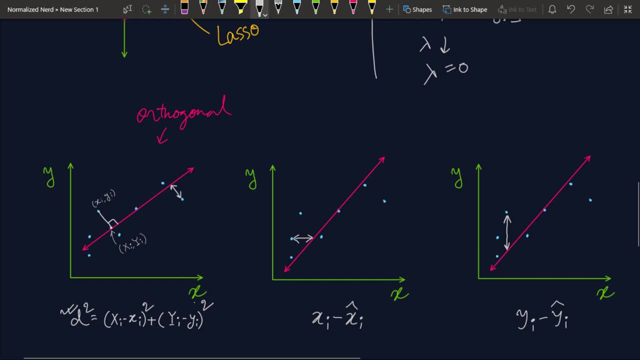 both the directions. You can just look at the formula here and you can just notice it, that we have both x-term and y-term. and, by the way, this capital xi and capital yi are just the foot of the perpendicular. All right, Now there is another variation of this, which is known as reduction. 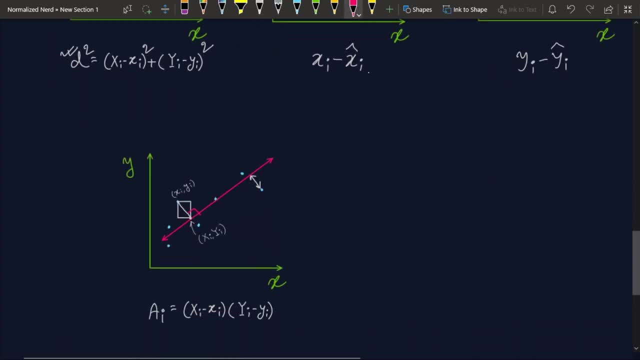 Reduced major axis regression. well, this concept is very similar to the above one. The difference here is, instead of calculating the d-square, we are just calculating the area extended by these two points. So to find the area, we just need to calculate the area of the rectangle, which can be easily. 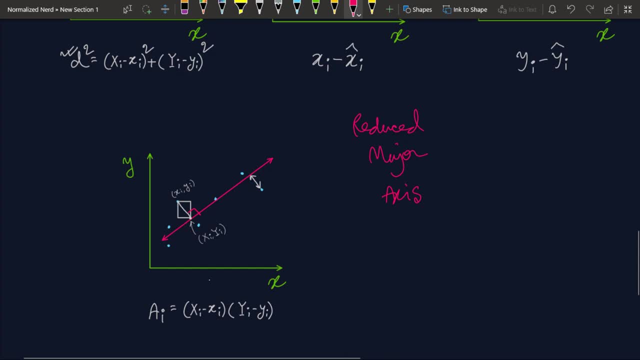 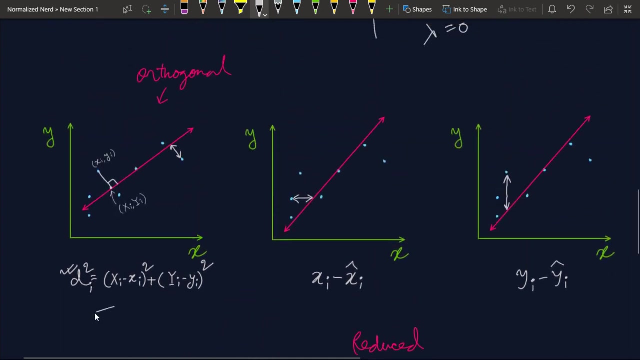 found by multiplying the x-error and y-error. Just to be clear here: what we are minimizing in reduced major axis and major axis regression is that in case of the major axis regression, we were actually minimizing the summation of d. i's okay, and the constraint in this minimization was our model, and let me just 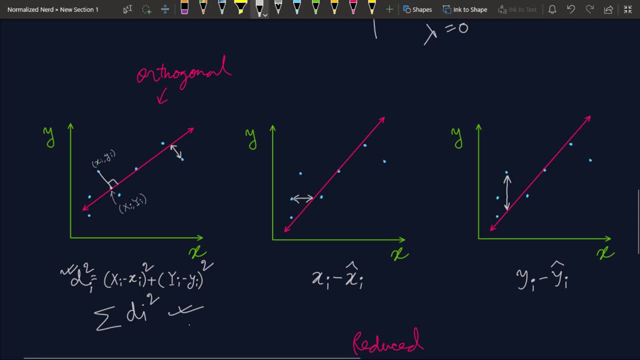 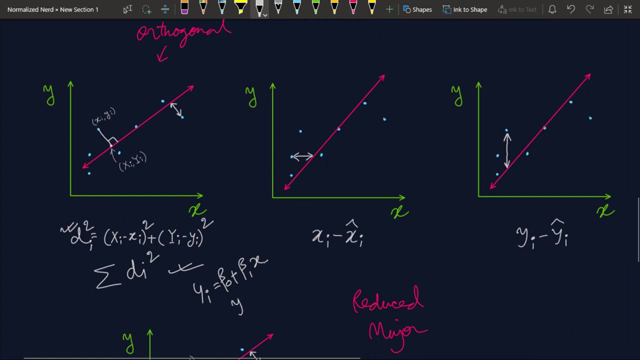 write the model here For convenience. I am working with only two variables, okay. So the model is: yi is equal to beta zero plus beta one x. okay, and if I just change the side here, you will notice that I will get yi minus beta zero minus beta one xi equal. 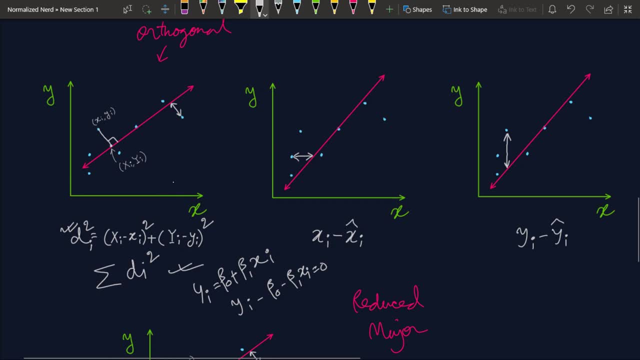 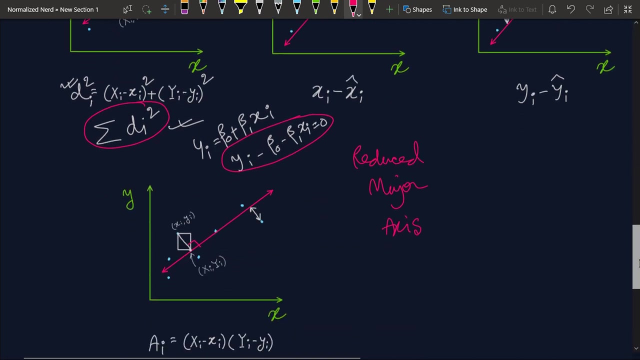 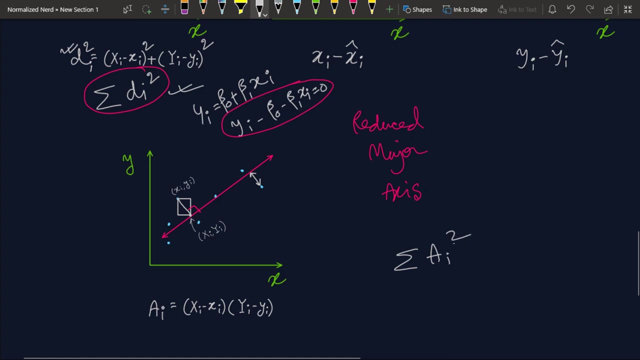 to zero. So the major axis regression is equivalent to saying that we are minimizing the d-square. Okay, So we are minimizing this term under the constraint, this equation, alright. and in case of the reduced major axis regression, we are minimizing this thing under the constraint. 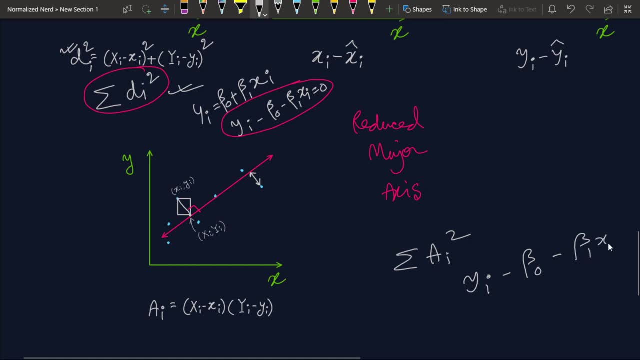 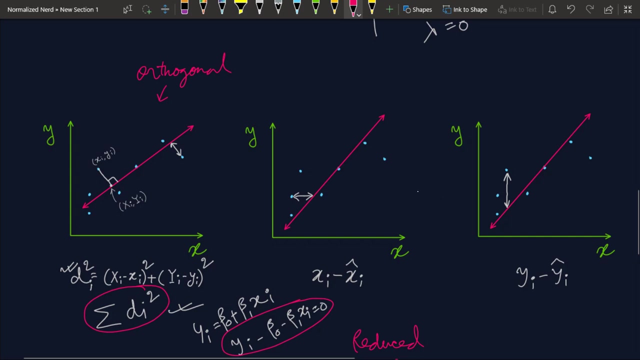 of this equation. So this is our minimization objective, Okay, And this is our constraint, Okay. So now I am going to answer. why would anybody want to use this orthogonal distance instead of this horizontal and vertical distances? Well, the main concept of this kind of error is that, to incorporate both the uncertainties, 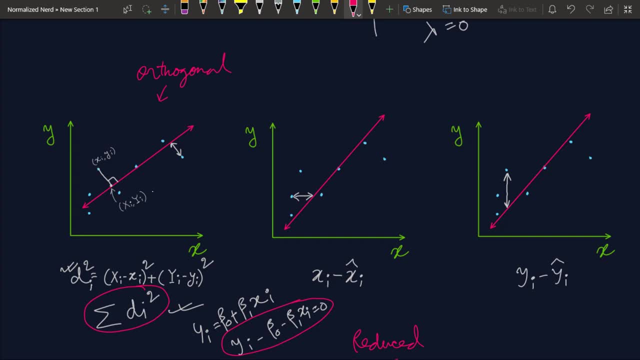 in y-axis and x-axis in our model. In other words, it may happen that in our model we are minimizing the summation of d? i. So what we are doing is that in our data we have uncertainties corresponding to both the independent variable, that is our x, and in the dependent variable, that is our y. 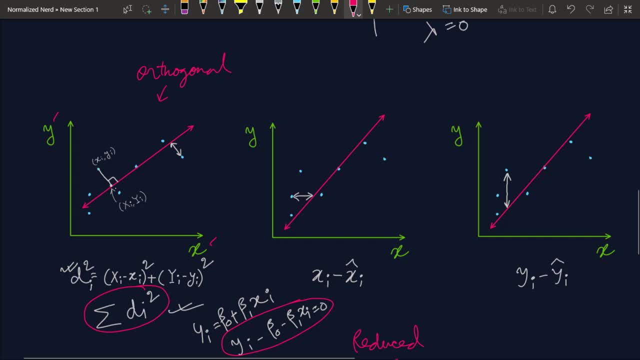 So to incorporate the errors, the uncertainties for both of them, we need to consider error in both the directions, and that is what we have done in orthogonal regression and reduced major axis regression. And I would also like to mention one interesting difference between this orthogonal regression: